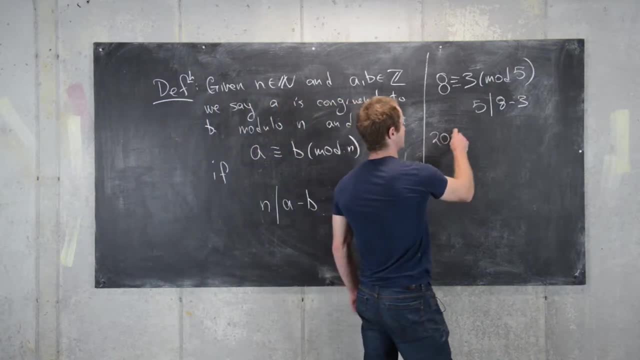 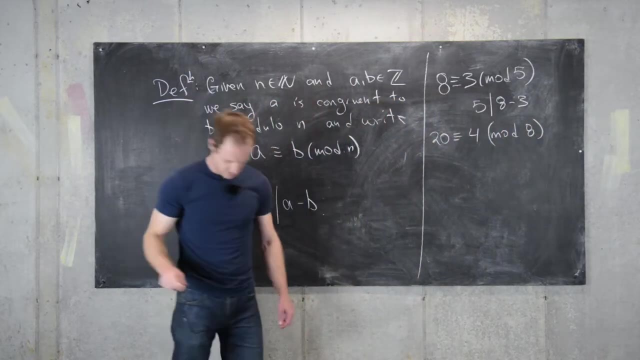 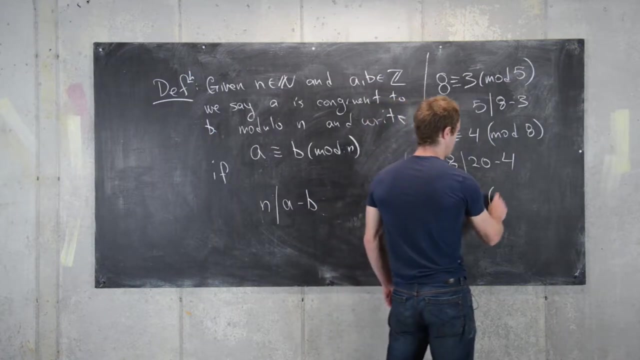 we're okay. And then 20 is congruent to 4 mod 8. And that's because 8 divides 20 minus 4.. 8 divides 16.. Okay, Okay, good, Now let's do one more. So 13 is congruent to negative 1 mod 7. And that's. 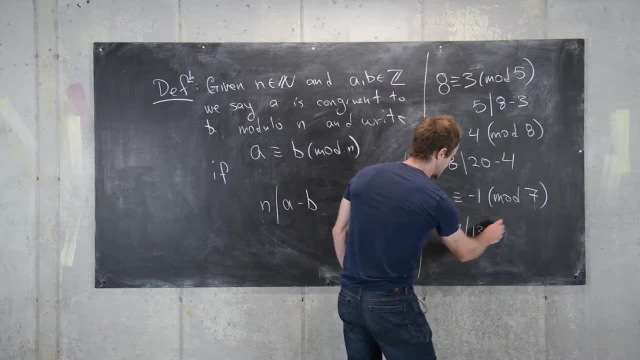 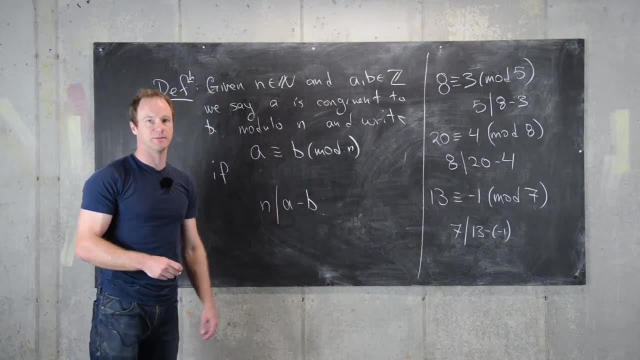 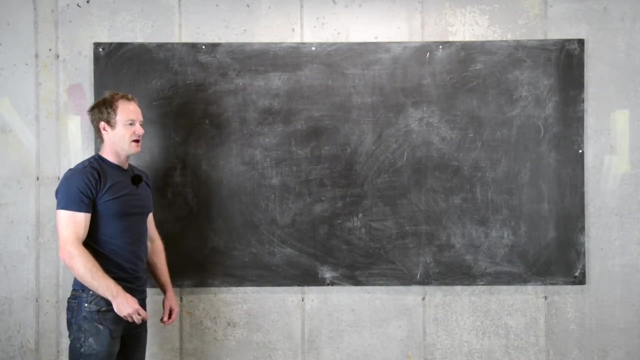 because 7 divides 13, minus negative 1.. So 7 divides 14.. Okay, good, So I'll clean up the board and then we'll look at some basic properties of this notion of congruence. Okay, this first property that we want to look at for congruence is that congruence. 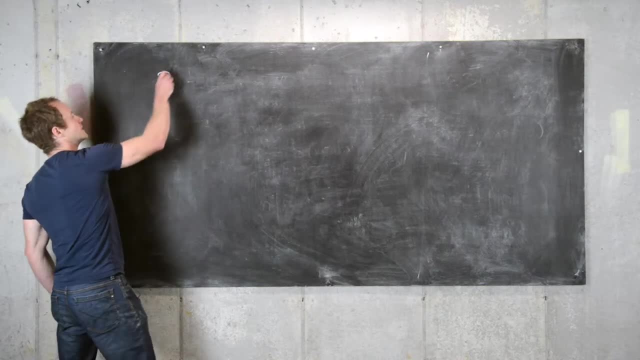 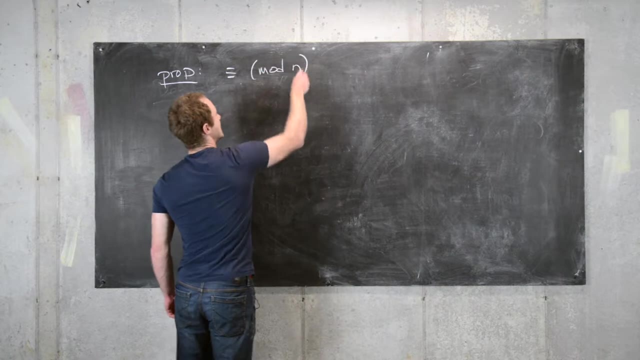 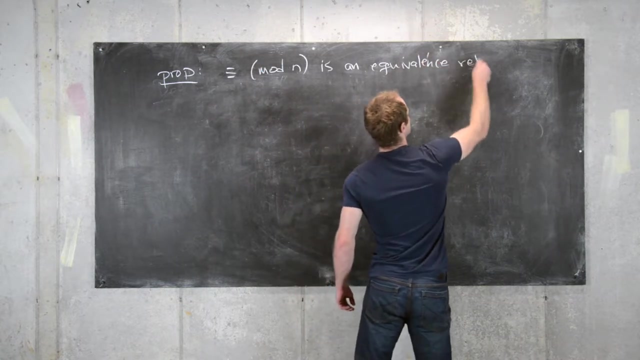 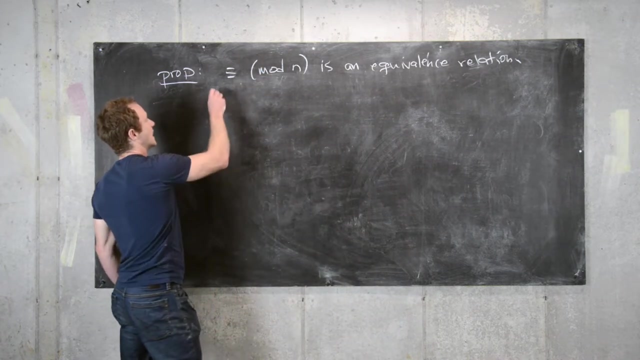 So congruence modulo n is an equivalence relation. So let's write that as a proposition. So we'll just do it in shorthand. So congruence mod n is an equivalence relation. So as a reminder what that is, we'll spell that out. So that is the following three things. 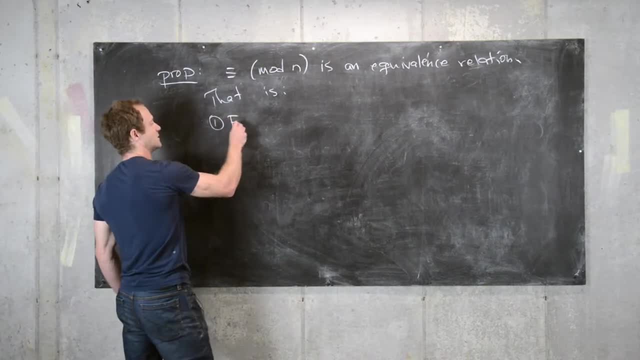 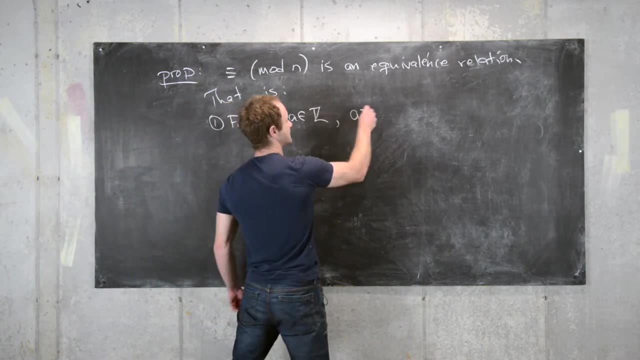 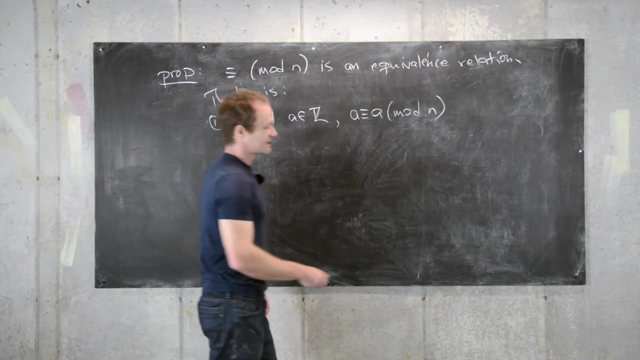 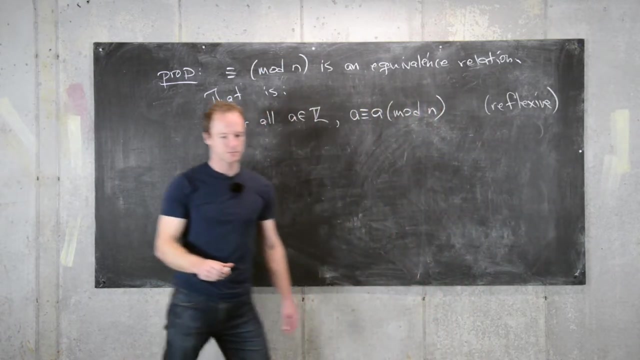 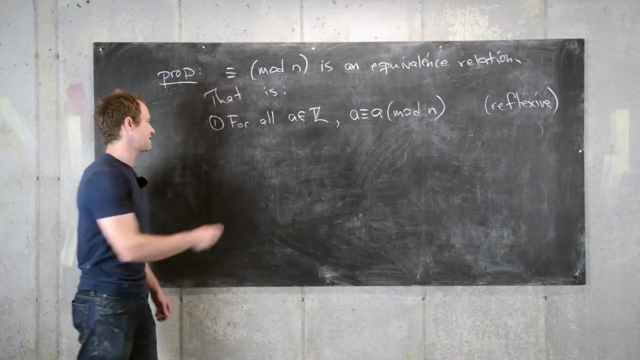 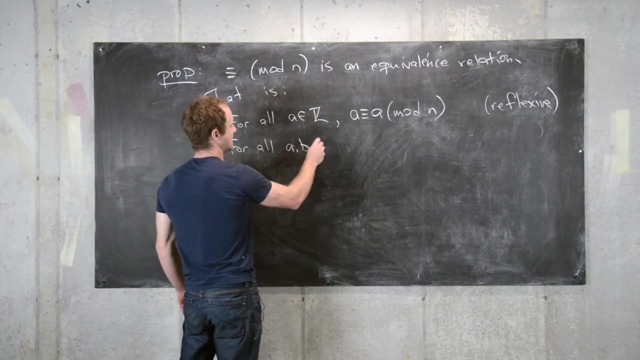 that are true. So the first one is for all integers a. A is congruent to itself, So A is congruent to a modulo n, And so this is reflexivity. Good, So the relation congruence mod n is reflexive. so then next we have for all a and b in integers. So if a is 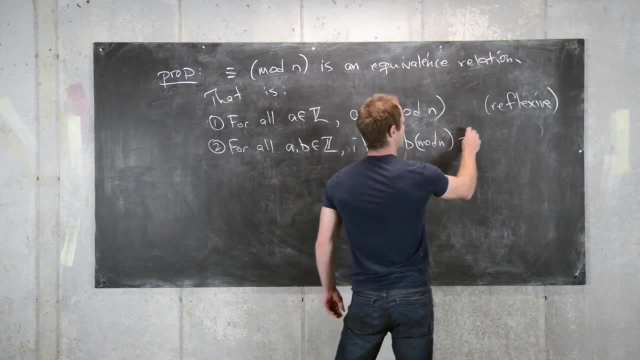 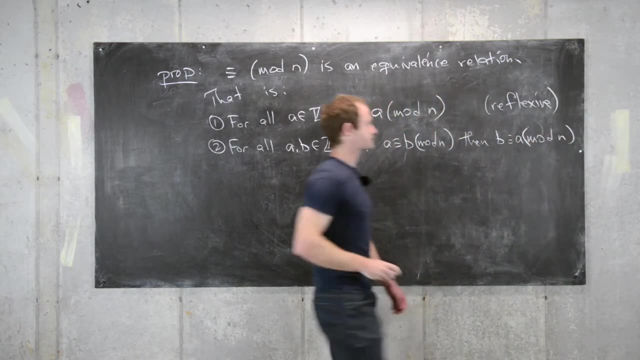 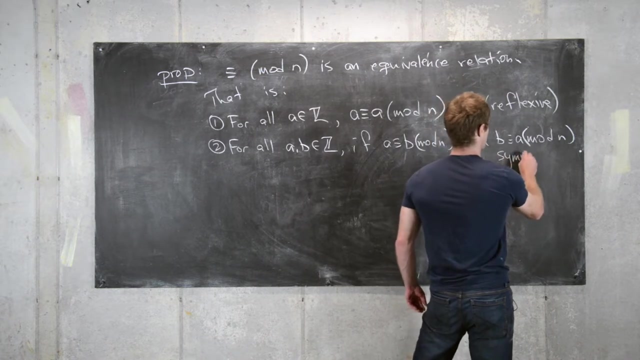 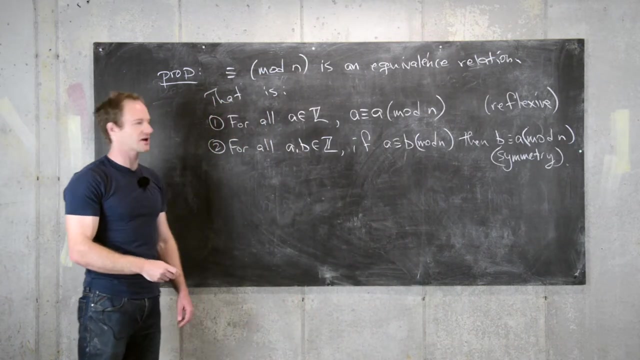 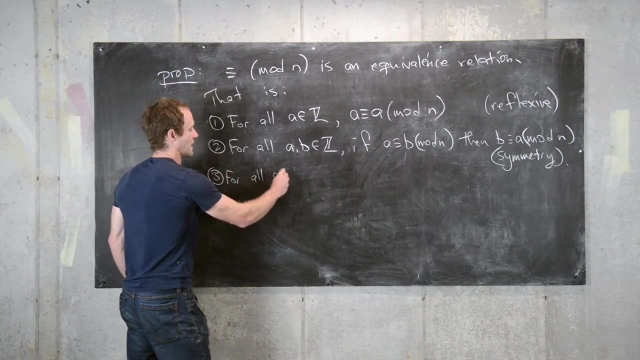 congruent to b mod n, then b is congruent to a mod n. Good, so this is a notice. this is the notion of symmetry, In other words, this relation of congruence: modulo n is symmetric, and then we have one more, and that is for all integers a. 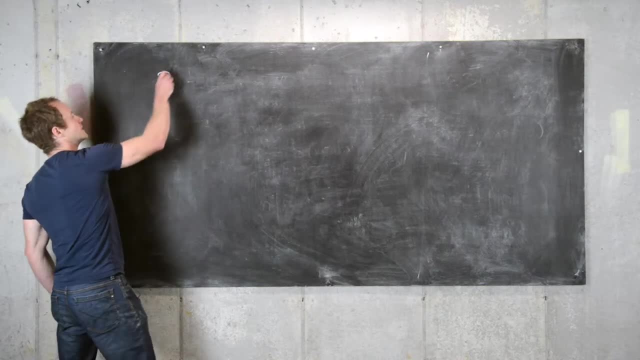 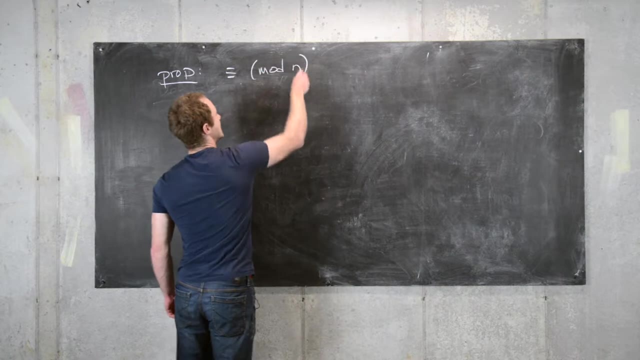 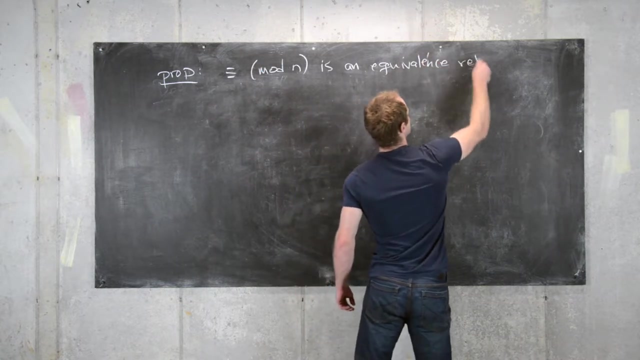 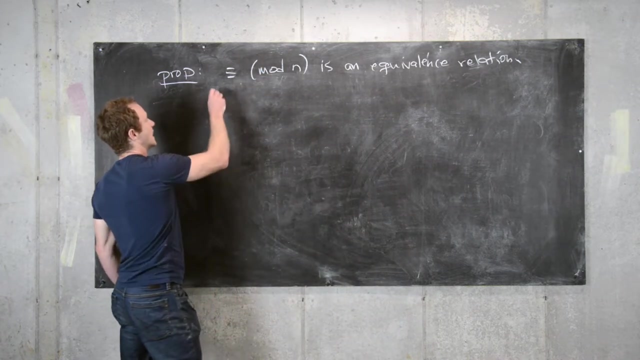 So congruence modulo n is an equivalence relation. So let's write that as a proposition. So we'll just do it in shorthand. So congruence mod n is an equivalence relation. So as a reminder what that is, we'll spell that out. So that is the following three things. 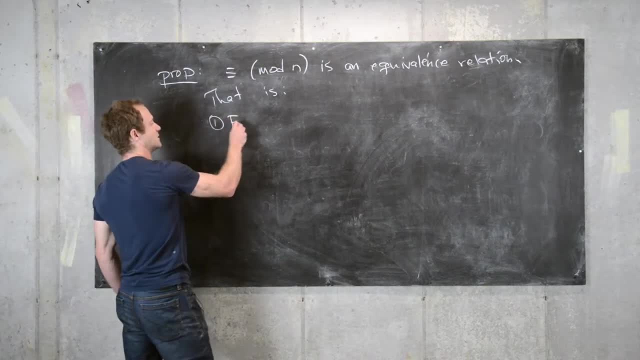 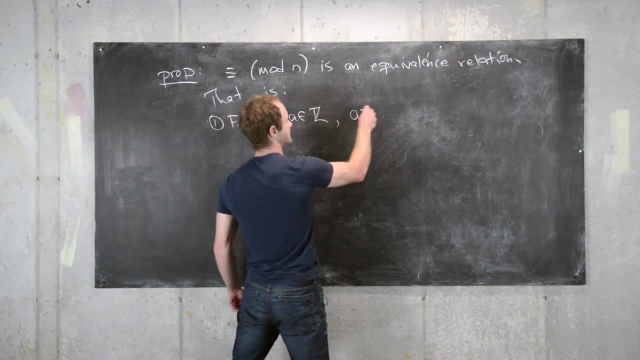 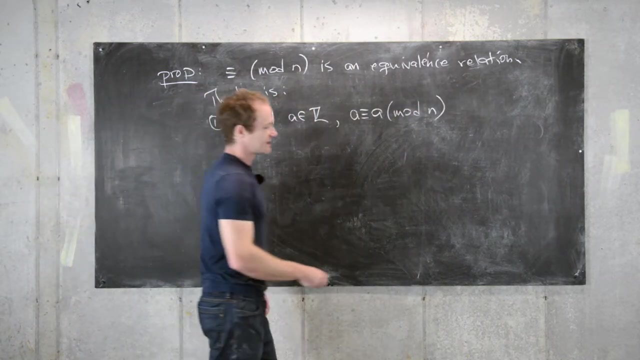 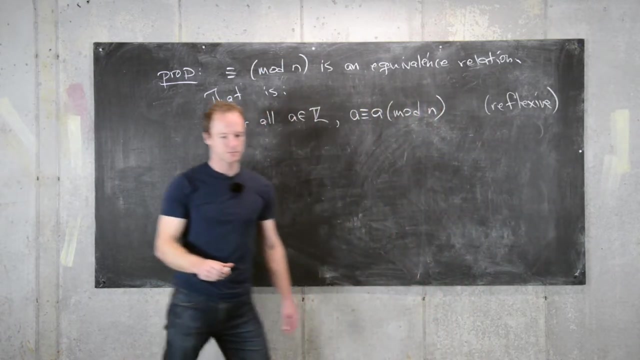 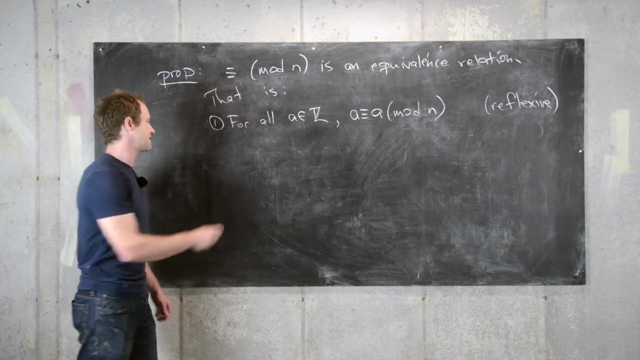 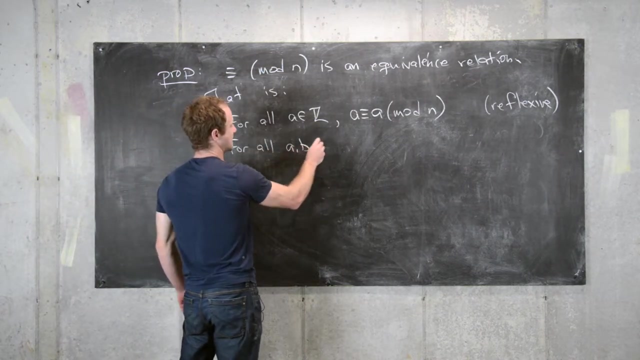 that are true. So the first one is for all integers a. a is congruent to itself. So a is congruent to a modulo n, And so this is reflexivity. Good, So the relation congruence mod n is reflexive. So then next we have for all a and b in integers. So if a is congruent, 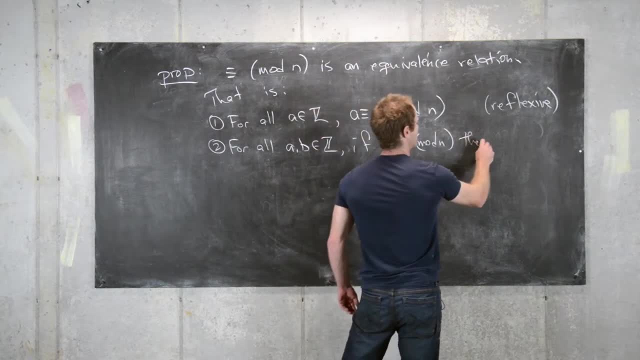 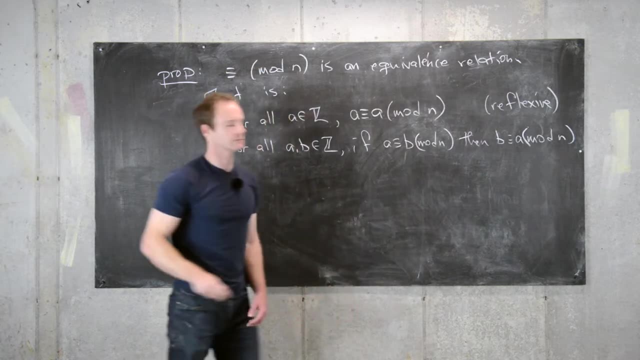 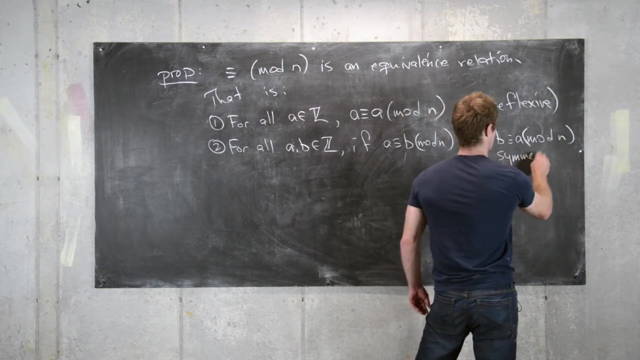 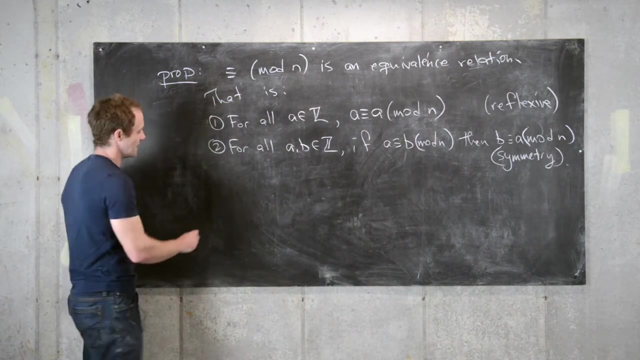 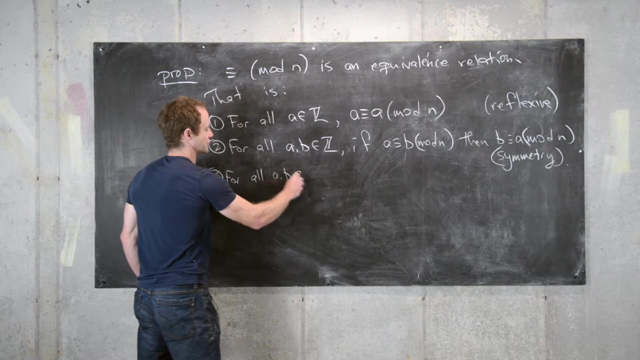 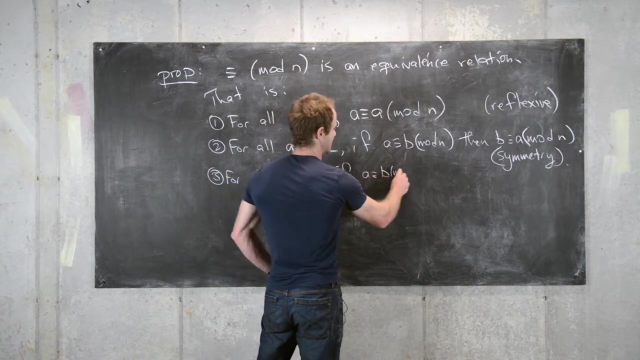 to b mod n, then b is congruent to a mod n. Good, So this is a notice. this is the notion of symmetry, In other words, this relation of congruence. modulo n is symmetric, And then we have one more, and that is for all integers, a, b and c. if a is congruent to b mod n and 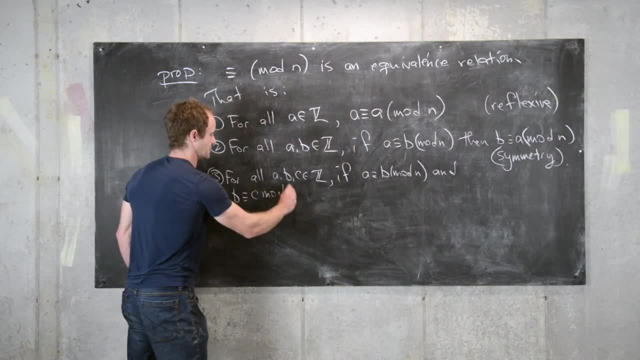 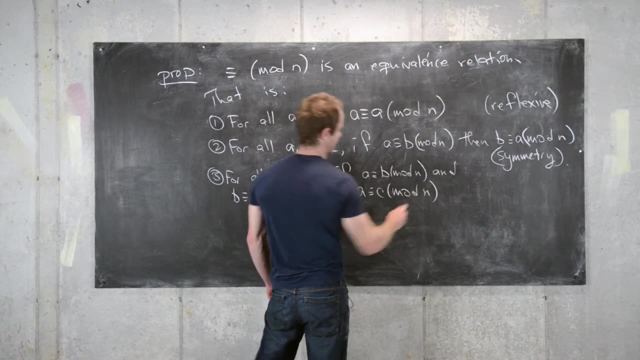 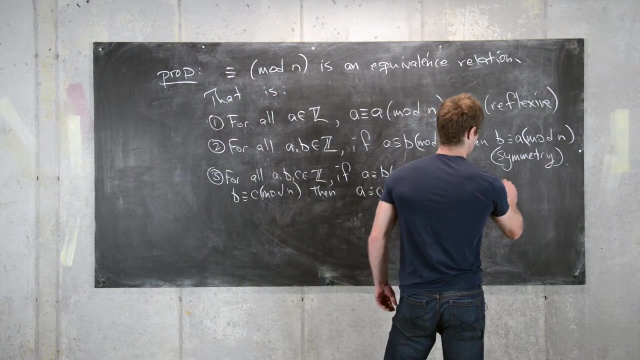 b is congruent to c- Good. So this is our first product. So we have a. a is congruent to b mod n and b is to C mod N. then A is congruent to C mod N- Good. So this is the notion of transitivity. 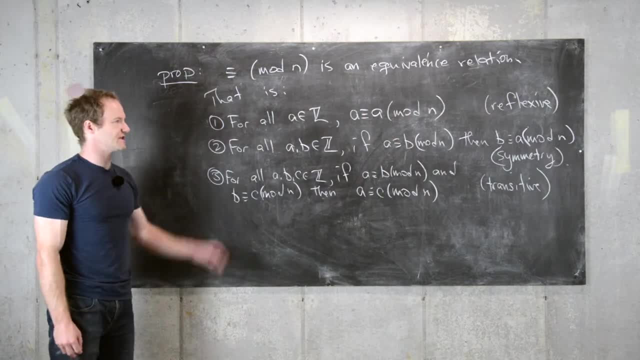 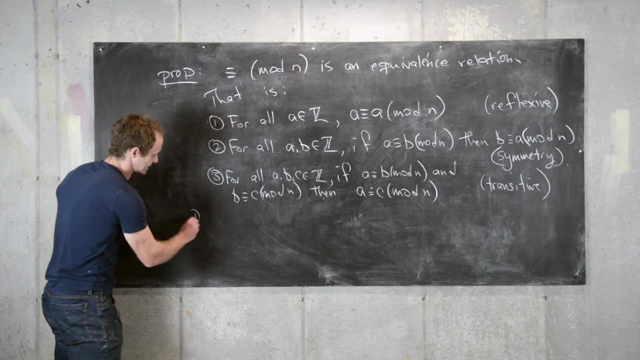 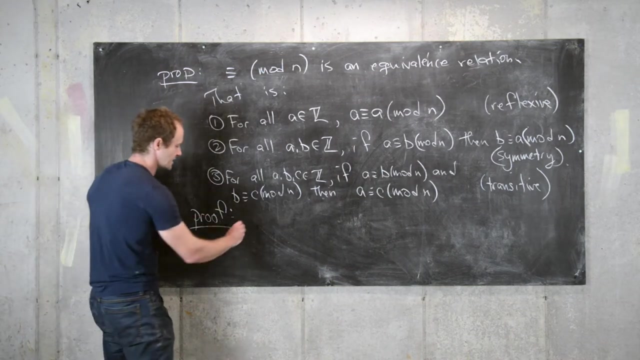 So this relation is transitive. So these three properties together make this equivalence modulo N and equivalence relation Good. So let's look at- we won't prove the whole thing, but maybe we'll prove part three real quick in the space that we have. So the proof of 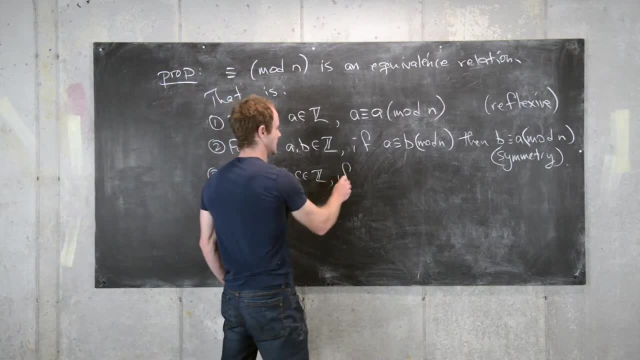 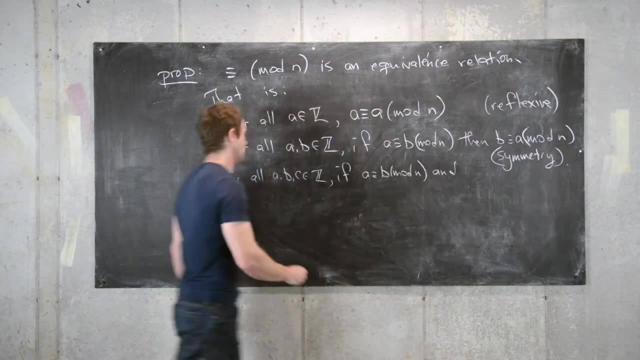 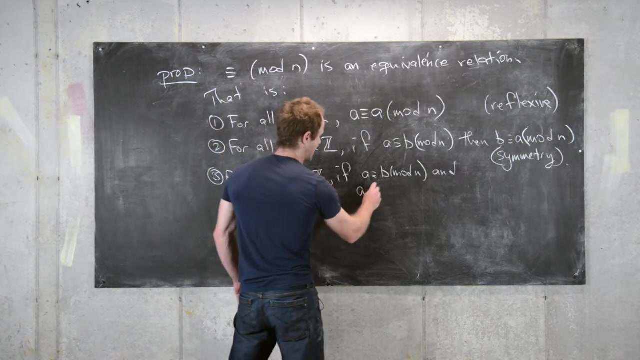 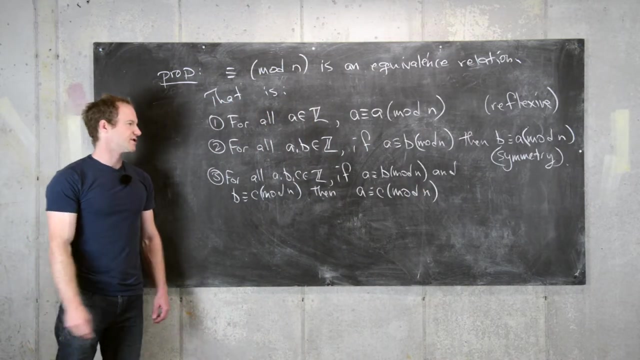 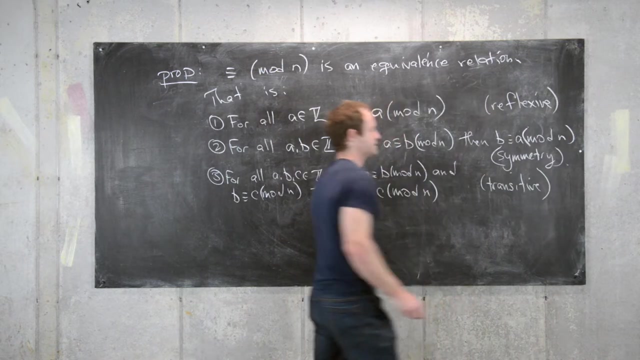 b and c. if a is congruent to b- mod n and b is congruent to c- mod n, then a is congruent to c- mod n. Good, so this is the notion of transitivity, So this relation is transitive. So these three 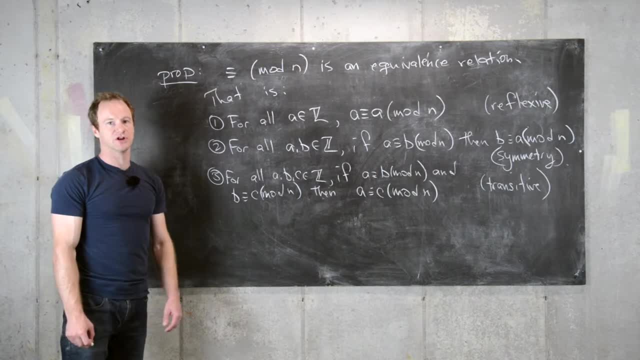 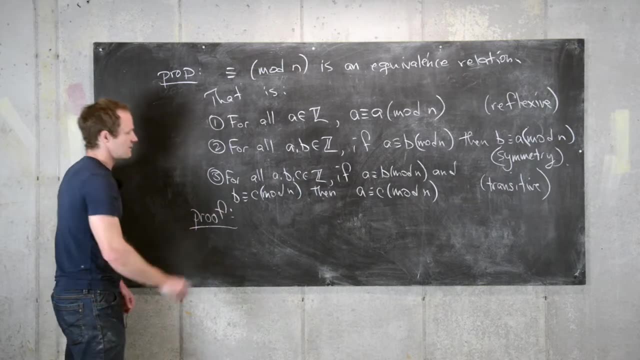 properties together make this equivalence modulo n an equivalence relation Good. so let's look at. we won't prove the whole thing, but maybe we'll prove part three real quick in the space that we have. So the proof of part three goes as: 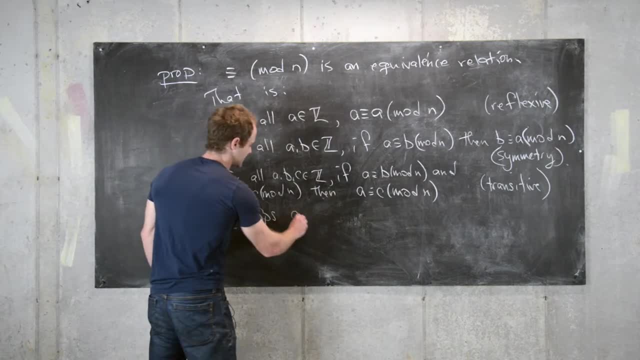 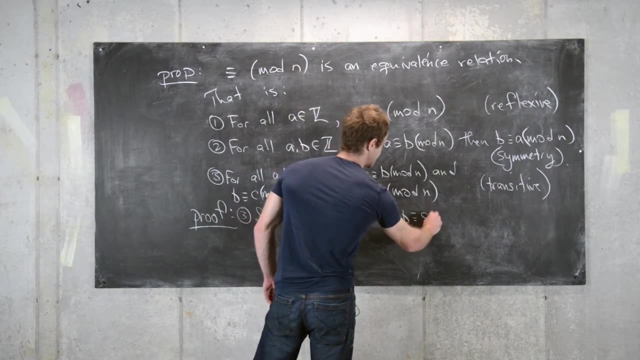 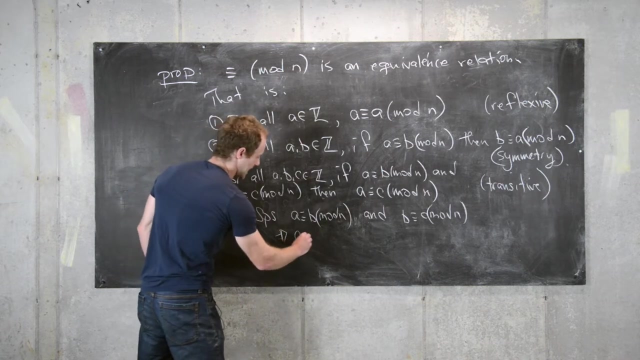 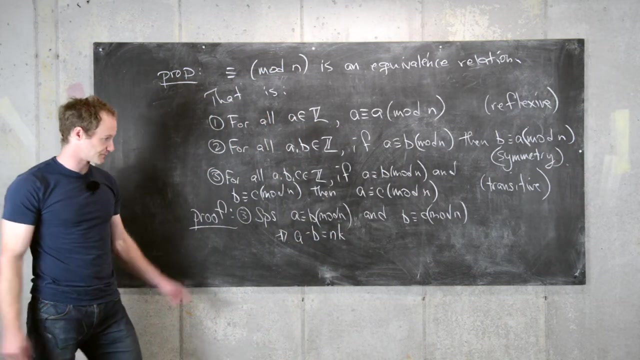 follows. So let's suppose that a is congruent to b mod n and b is congruent to c mod n. Good, so that tells us that a minus b equals n times k. for some integer k, because, recall, this means that n divides a minus. 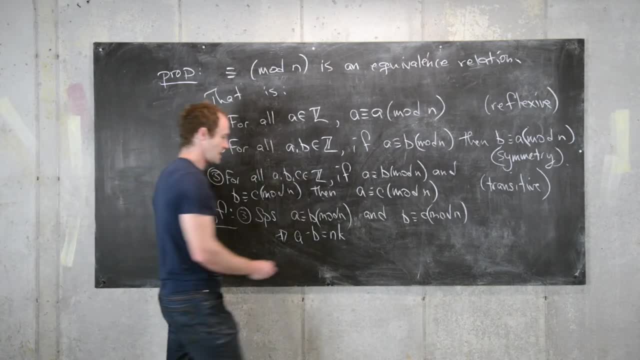 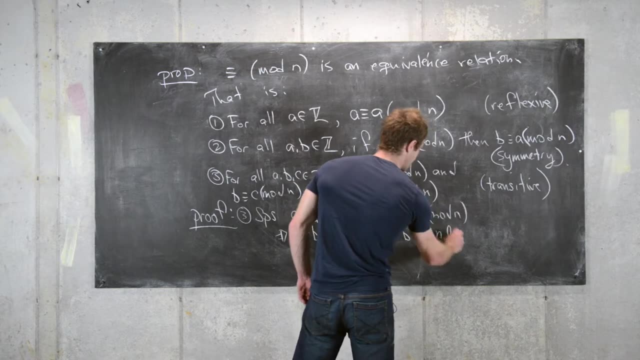 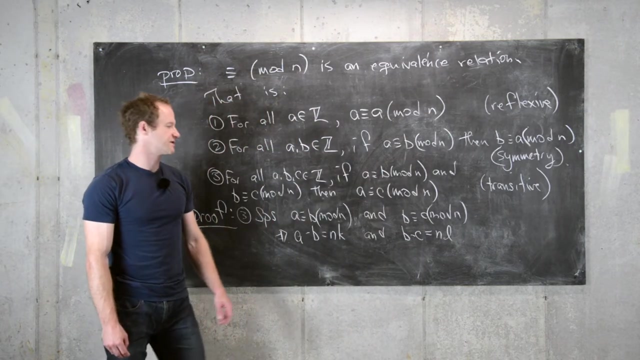 b. but that means that a minus b is a multiple of n, and b minus c is equal to n times l. for some integer l again, because n divides b minus c, and so if n divides b minus c, b minus c is a multiple of n. So if n divides b minus c, b minus c is a multiple of n. so 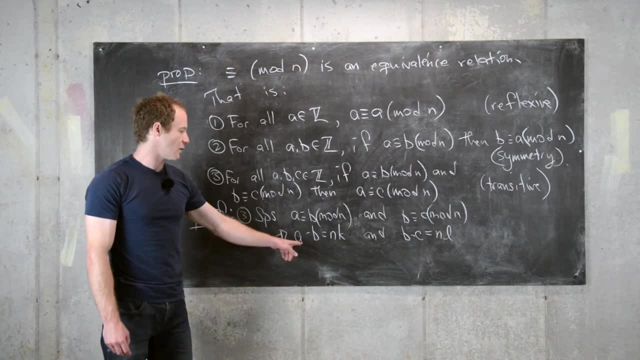 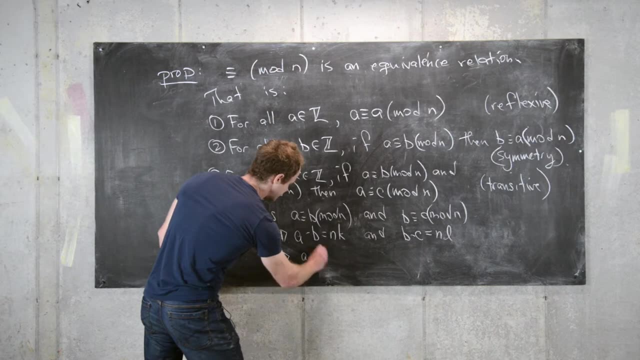 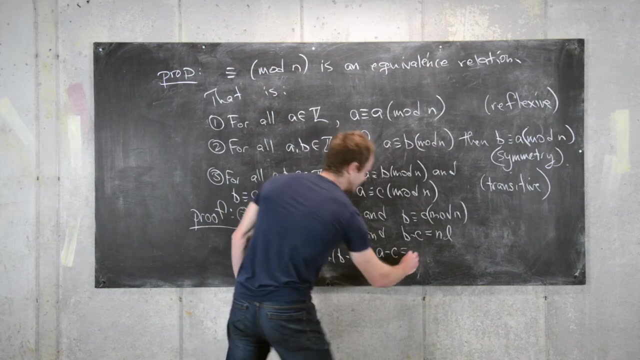 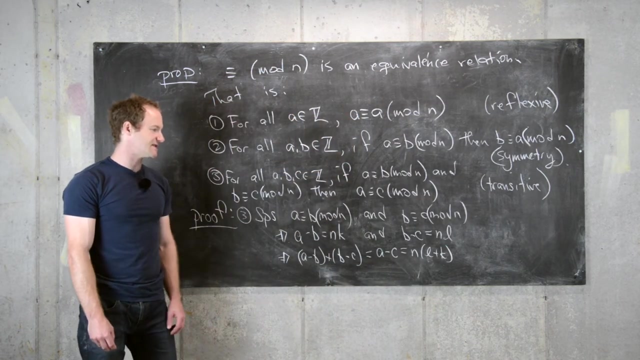 we can write it as follows: Good, and now what we can do is add this equation to this equation, So that'll give us a minus b, plus b minus c. that's equal to a minus c, and that's equal to n times l plus k. So what we have is a minus c, is a multiple of n. but 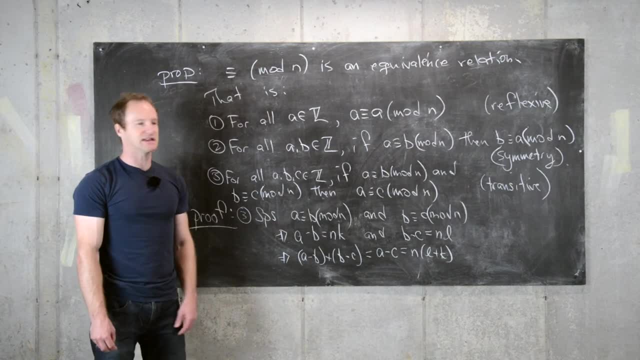 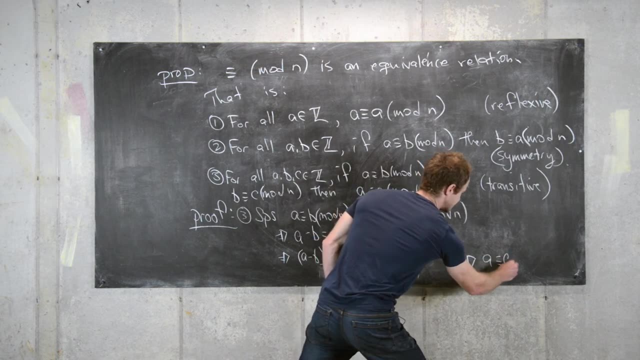 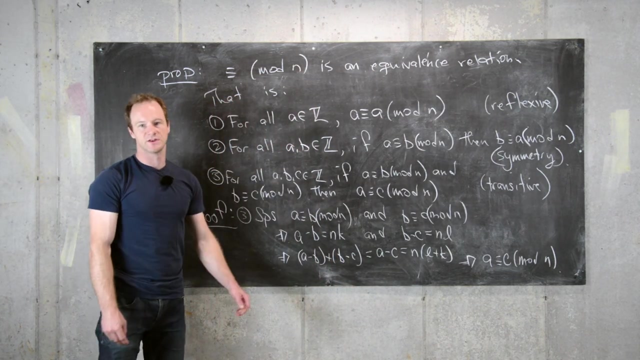 that means that n divides a minus c, But in turn that means that a is congruent to c mod n. So we'll finish it off. a is congruent to c mod n. Okay, good. So that's the end of the video. We'll look at some more properties. in the next video. 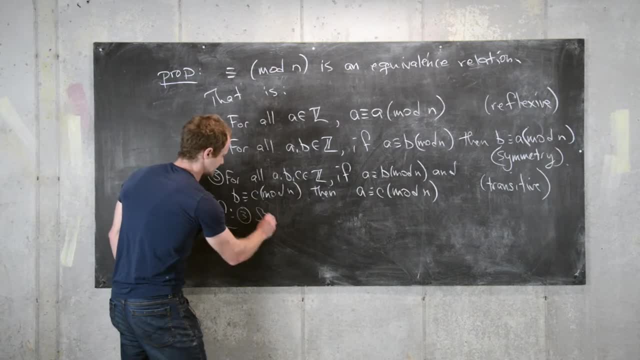 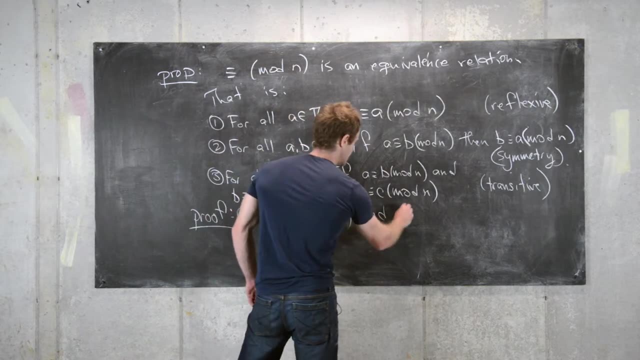 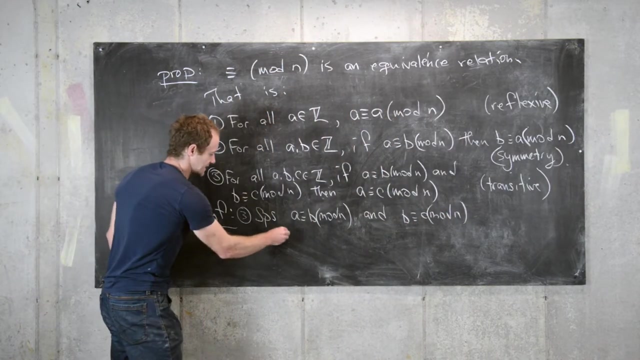 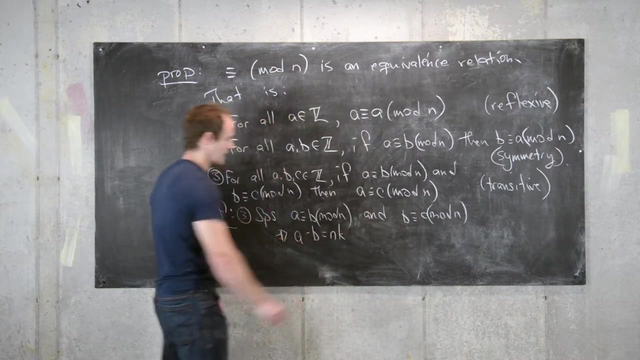 part three goes as follows: So let's suppose that A is congruent to B mod N and B is congruent to C mod N. Good, So that tells us. So that tells us that A minus B equals N times K, for some integer K, because recall this. 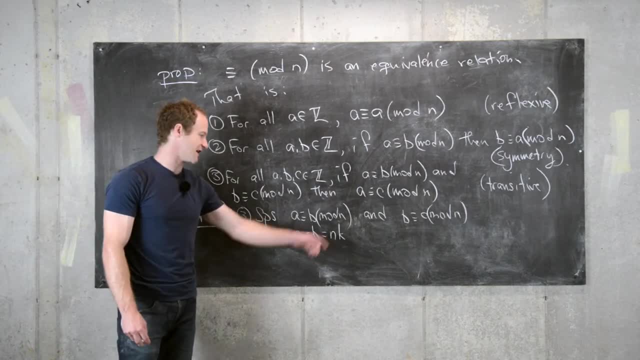 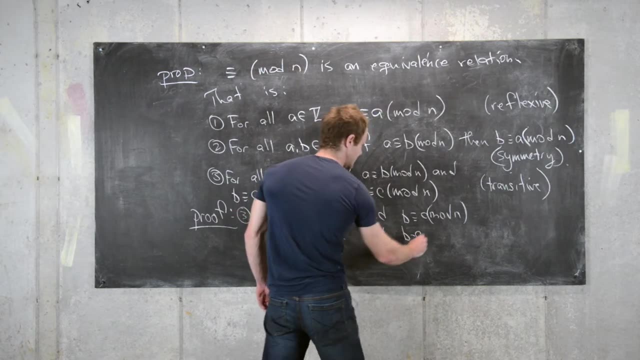 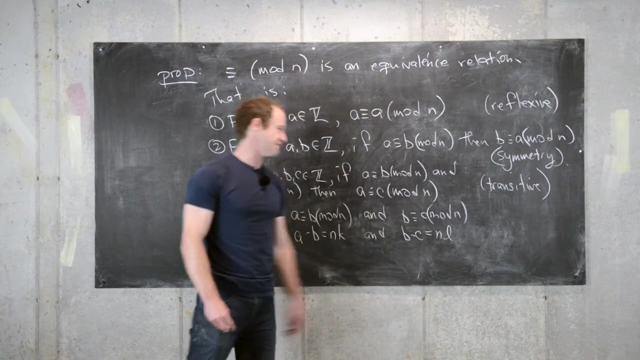 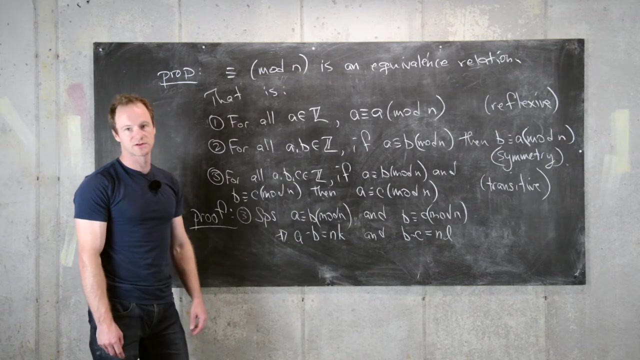 means that N divides A minus B, but that means that A minus B is a multiple of N, and B minus C is equal to N times L for some integer L again, because N divides B minus C, And so if N divides B minus C, B minus C is a multiple of N. so we can write it as follows: Good, 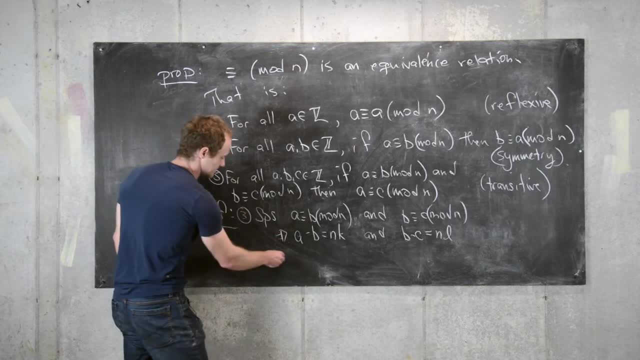 And now what we can do is add this equation to this equation, So that will give us A minus B plus B minus C. That is equal to A minus C, and that is equal to N times L plus K. So what we have is A minus C is a multiple of N plus Z minus P, minus X minus X N. So these 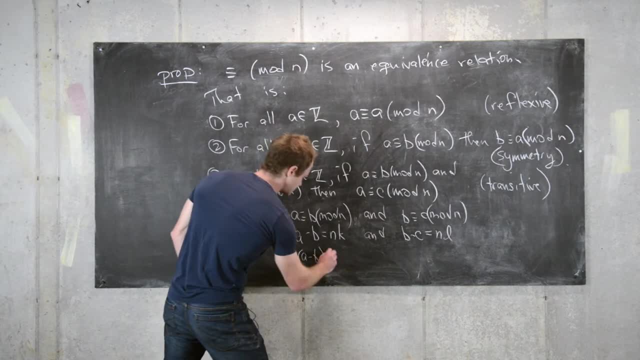 are ionic 2 random numbers in the ragging system. Now this is going to take us down to how many of these, was our answer. So how many of these numbers do we need to save? Well, we put 3 in here and we have 11 in here. So if we put our first number in here, 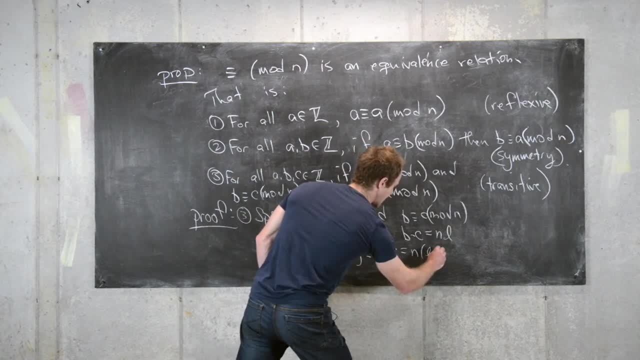 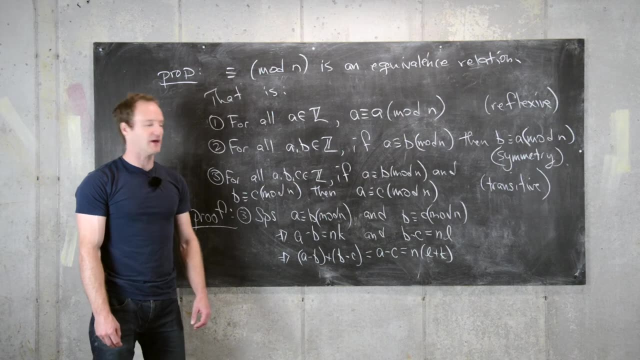 we will see what our answer is of 25.. We don't have anything more to do than solve now One of these terms we need to learn. B minus B equals C. so if we combine all So what we have is A minus C, is a multiple of N. 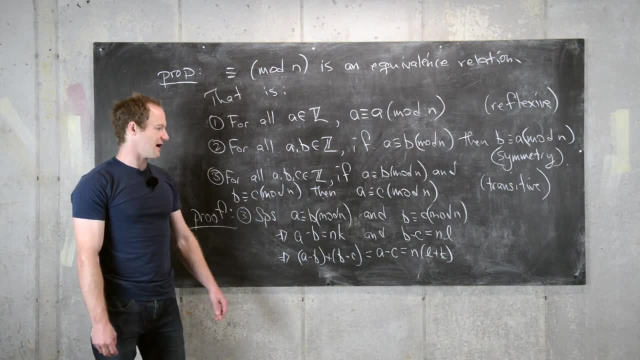 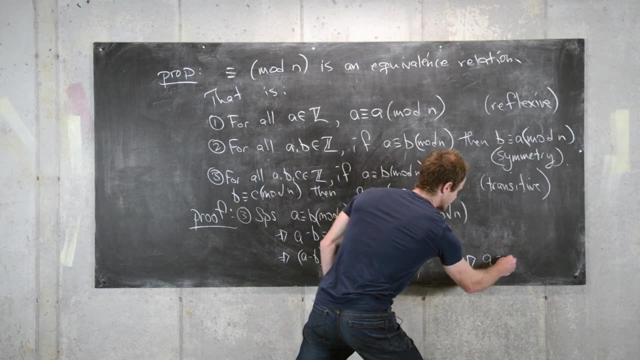 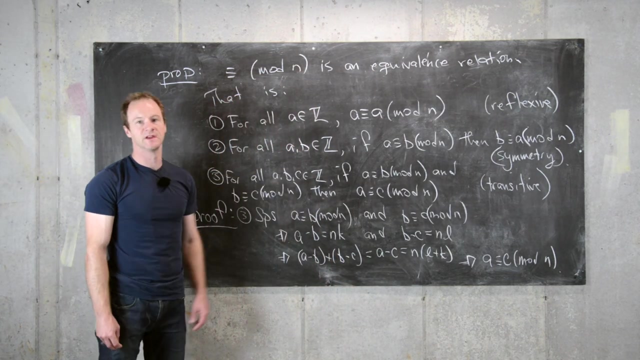 but that means that N divides A minus C, but in turn that means that A is congruent to C mod N. So we'll finish it off. A is congruent to C mod N. Okay, good. So that's the end of the video. We'll look at some more properties in the next video. 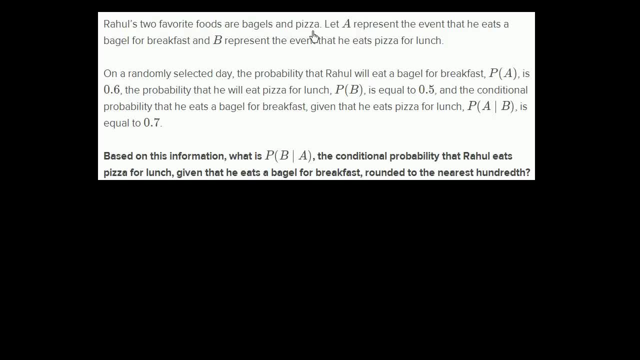 Rahul's two favorite foods are bagels and pizza. Let A represent the event that he eats a bagel for breakfast and let B represent the event that he eats pizza for lunch. Fair enough, On a randomly selected day, the probability that Rahul will eat a bagel for breakfast?